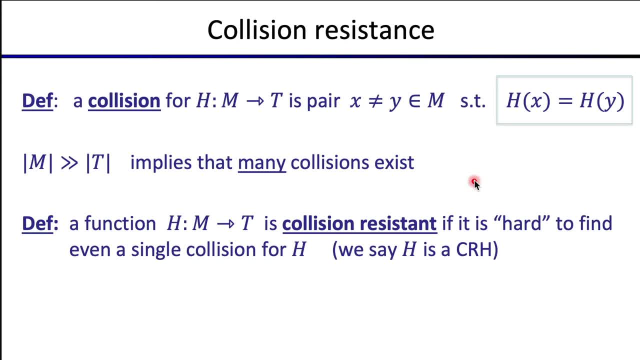 The point of a collision resistant hash function is that, even though there is a huge number of possible collisions, it's hard to point to even one explicit collision. Yeah, it's hard to find even a single pair- x, y- that happens to collide. for the hash function h. 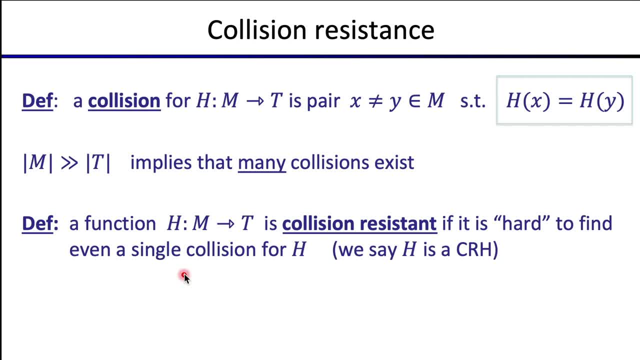 So if that's true, if the hash function h has this property, we say that h is collision resistant and we'll write that h is a CRH- CRH just stands for collision resistant hash. So you might be wondering: well, what's an example of a collision resistant hash function In the canonical example? 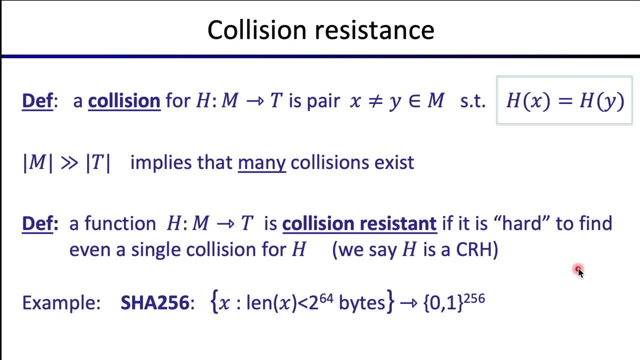 is this hash function called SHA-256.. This is a fixed hash function that's actually specified in a federal standard. What it does is it takes an arbitrary amount of data, well up to 2 to the 64 bytes, so potentially megabytes, even petabytes of data, and it always maps them to a 256-bit output. 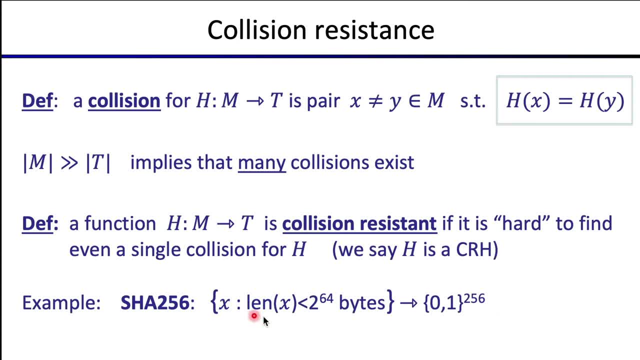 which again means 32 bytes. Okay, so again, huge amounts of data come in, 32 bytes come out, And the function is collision resistant, which means that it's difficult to find two distinct messages that happen to map to the same 32-byte digest. 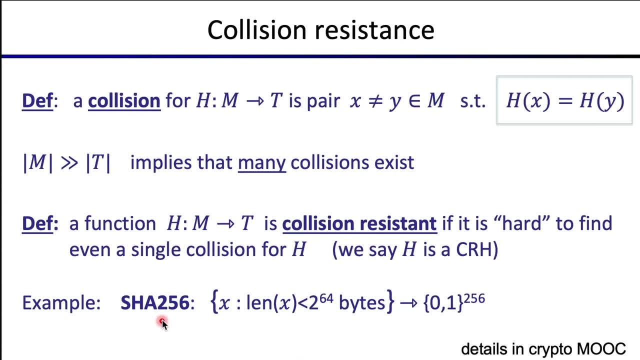 Now, if you want to see how collision resistance is built and how SHA-256 works- I'm not going to describe that here, but I would refer you to my crypto MOOC- You can take a look at the lecture on collision resistance and there's a lot of information there on why the hash function is built the way it is and how these collision resistant hash 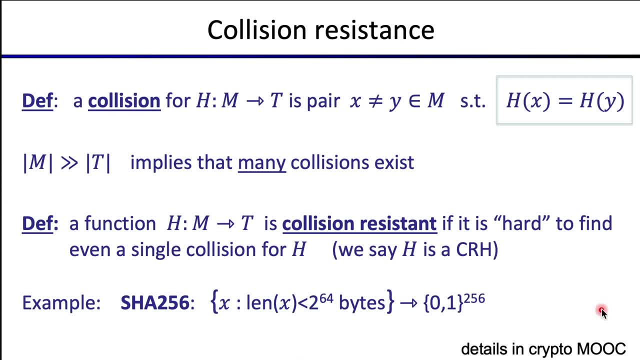 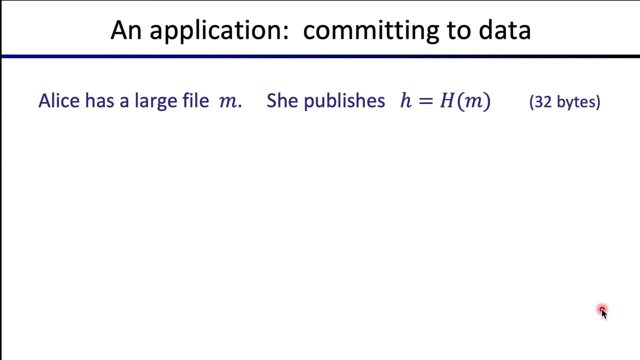 functions actually operate. But for now we'll take SHA-256 as a given And we'll assume it's collision resistant. So there are many applications for cryptographic hash functions. They're useful in proof of work consensus, which we're not going to talk about here. 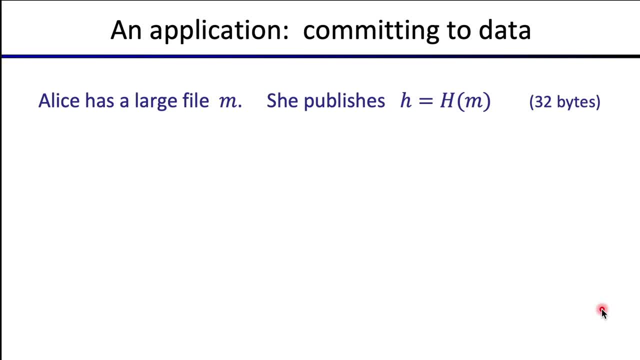 Instead, I want to talk about an application for collision resistance that has to do with committing to large amounts of data. Okay, so imagine Alice has a file, or maybe a message, which will denote by M, So she has a fairly large amount of data. 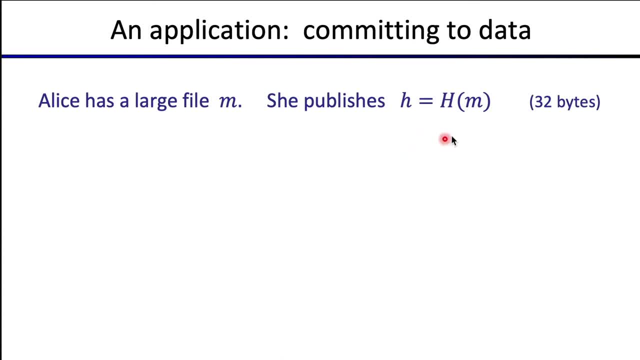 And what she will do is she will commit to this data by publishing a hash of the message M. So the hash is only 32 bytes. So it's a very, very short commitment to possibly megabytes of data, And we want to say that this little digest H actually commits her to the message that she just committed to. 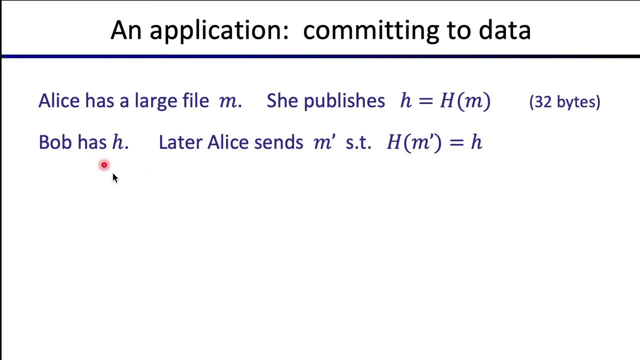 So what does that mean? Suppose Bob actually has the commitment. So Bob has the little H output of the hash function And then later Alice sends to Bob the message M prime, claiming that this is the message that she actually committed to. Okay, well, Bob can check that H of M prime is equal to little h. 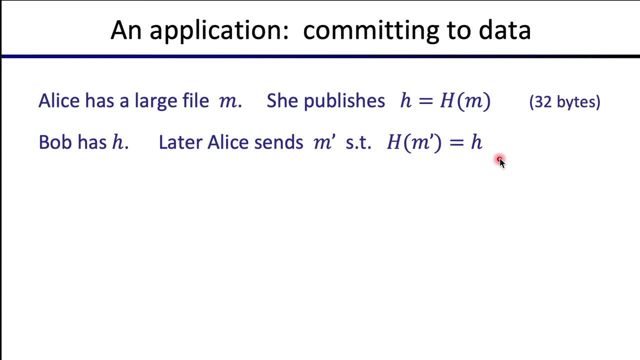 And the claim is that if the hash function is collision resistant, then if this equality holds, then Bob is convinced that the message M prime really is the message that Alice committed to. Let's say that more precisely: If H is a collision resistant hash and H of M prime is equal to little h, 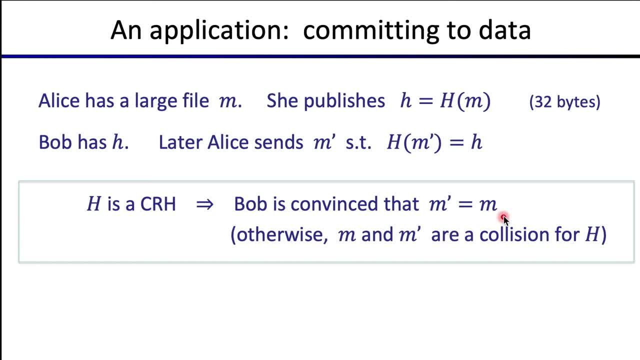 then Bob is convinced that M prime is equal to M. Yeah, Why is that true? If somehow Alice was able to find M and M prime such that H of M is equal to H of M prime, but M is not equal to M prime, well, that would be a collision for the hash function H. 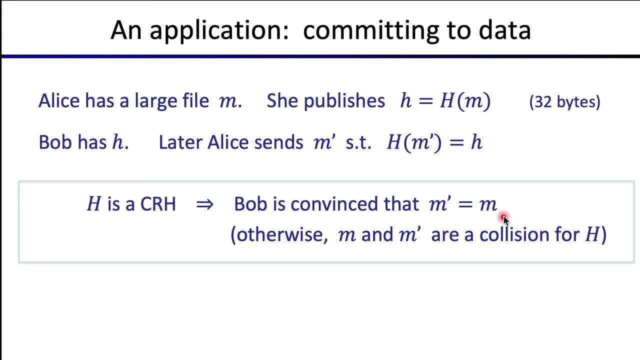 But because we assumed H is collision resistant, that's going to be difficult for her to do. So what this means is again that if Alice publishes a collision resistant hash of her message M, then that little h, that little hash value little h. 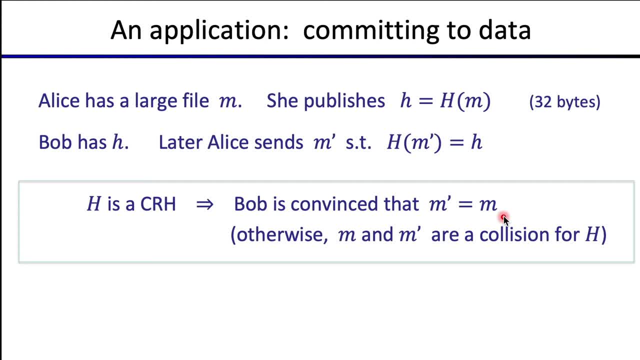 is committing her to the message M, And the only way that she can find an M prime that maps to little h is if M prime is equal to M. Okay, So we say that this is what's called a binding commitment to the message M. 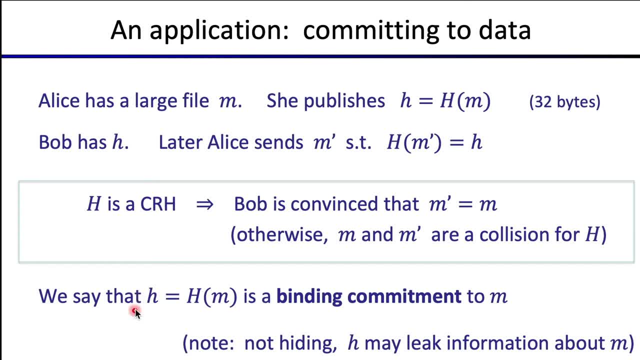 because once Alice publishes little h, she can no longer change her mind about little m. Now, one thing that I want to point out is that this sort of commitment is not a hiding commitment, in the sense that the hash of the message M might actually leak information about M. 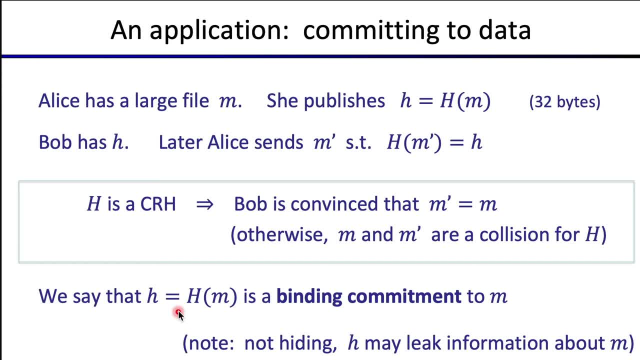 Yeah, Yeah. And so this is not a hiding commitment. it's not hiding the message, but it is binding in the sense that once Alice commits, she can no longer change her mind about the contents of the message M. So let's look at a more interesting application. 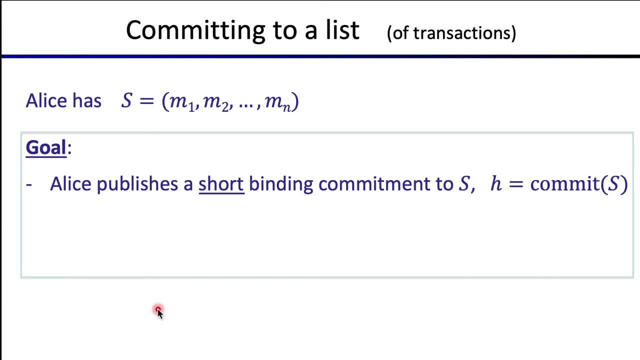 which is committing to not just a single message but in fact a list of messages. And just looking ahead, the list of messages we're going to be interested in committing to is going to be a list of transactions in a block. So suppose we have M1 to Mn. 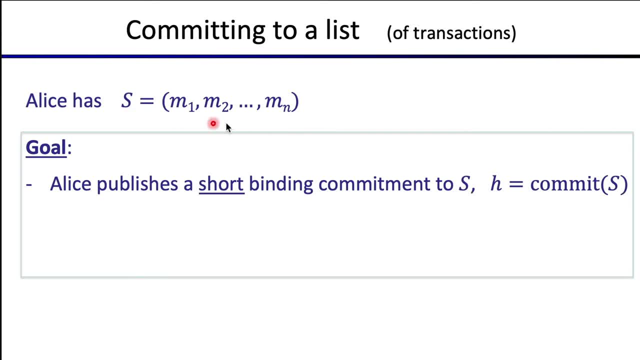 These are N different messages That let's say they form a list and we'll call this list S. Now our goal is to build a commitment scheme with the following property: So Alice is going to publish a short binding commitment to S. 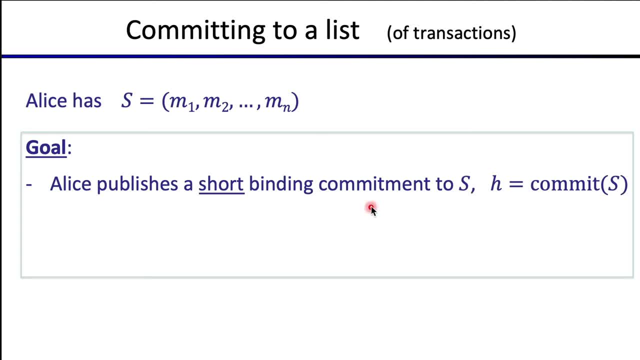 Okay. so once she publishes the commitment, she can no longer change her mind about the committed messages, And this commitment is going to be this short digest, So it again has to be just 32 bytes. Now, again, as before, Bob is going to obtain this commitment value. 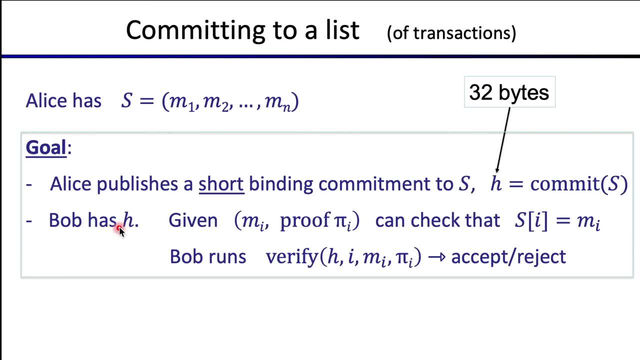 So he's going to, He's going to obtain little h And then later on, Alice would like to prove that the message at position i is equal to Mi, And to do that, she's going to send to Bob the message Mi. 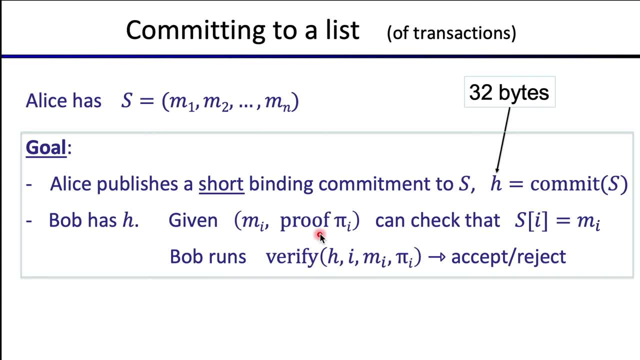 along with some sort of a proof, which we'll call pi i. Pi stands for proof That this proof, pi i will convince Bob that the message at position i, the committed message at position i, is really Mi. Yeah, so S of i is equal to Mi. 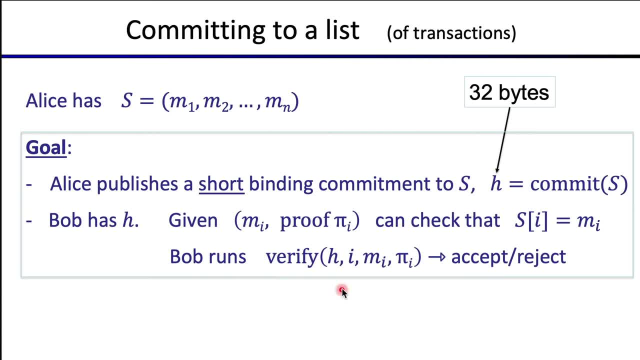 To do that, Bob is going to run through some verification algorithm. The verification algorithm is going to take the commitment, the index, the candidate message, Mi and the proof and is either going to accept or reject that proof. From a security point of view, 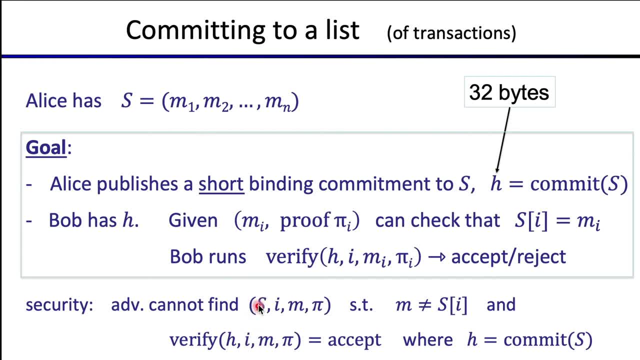 we'd like to say that an adversary cannot find a list S, an index i, a message M and a proof pi such that M is not equal to S of i, and yet the proof is accepted by the verification algorithm. Yeah, this should be hard. 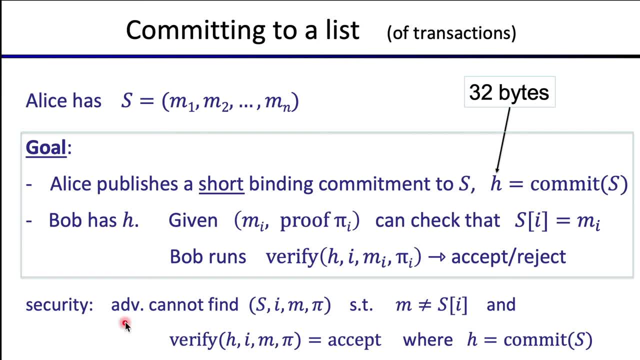 And if that's true, then we say that this is a valid commitment to a set that allows opening of elements in this set. So how do we do this? So how do we commit to a set and then later open up only one element in the set? 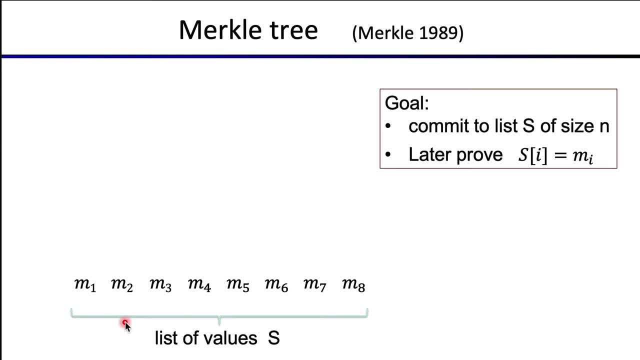 using a very short proof. So the trick to do this is what's called a Merkle tree. Okay, this is due to Ralph Merkle, already back in 1989. So it's an old idea, but this idea is so important that it's now used everywhere in the blockchain space. 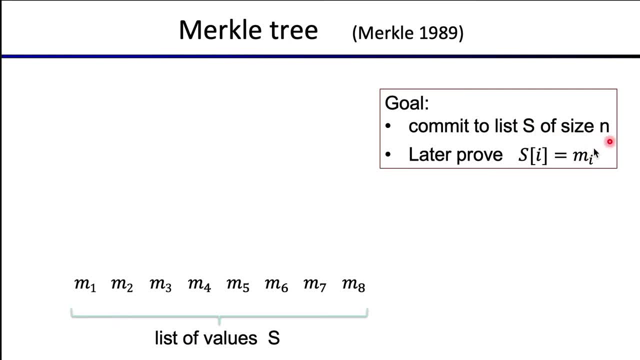 So let's see how this works. So we're going to commit to a list of sets of size N here. we'll assume we have only eight elements, so N is equal to eight. We're going to commit to these eight messages. 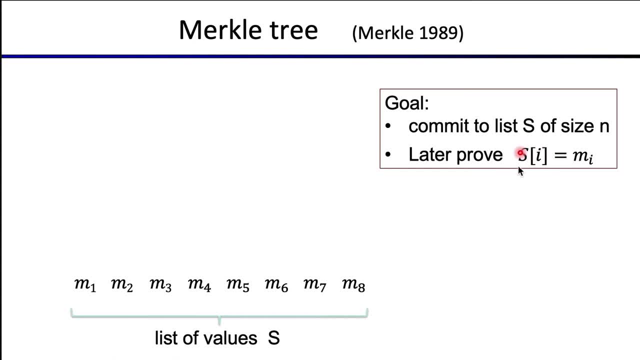 And then we want to be able to later prove that entry number i in the list is equal to M i. So the way we're going to do that is by committing, by forming a Merkle tree, and we're going to produce this short commitment H. 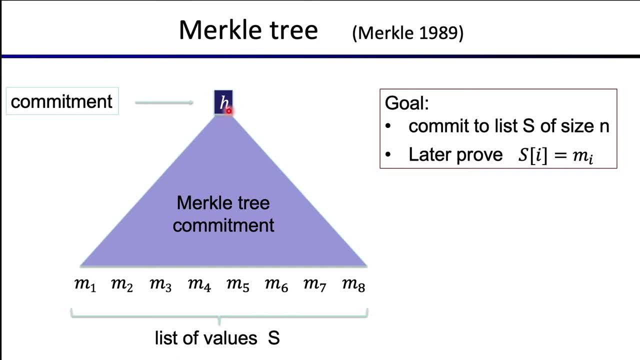 which is again just 32 bytes, nothing more. Very, very short commitments. even though we might be committing to a million elements where each element is a megabyte long, The commitment overall, it's just 32 bytes, And the way we do that is basically. 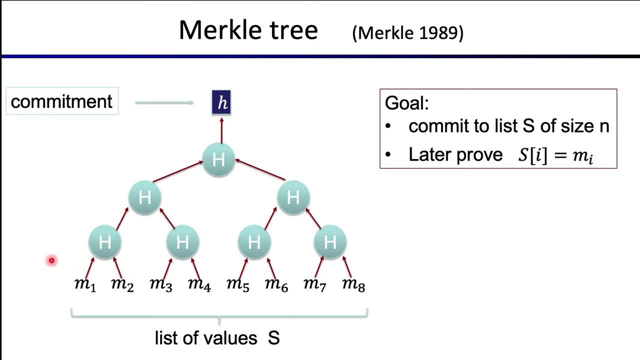 by forming this Merkle tree. So a Merkle tree is basically a tree of hashes, where you can see that we're hashing all bottom pairs, Then we're hashing all hashes. Yes, so that's how we get the second layer of hashes. 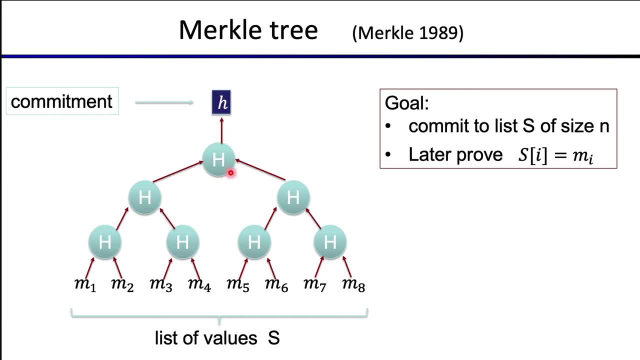 Then we hash again, all hashes, And then finally, once we're done, to a single hash, that's going to be the final commitment that we're going to send over to Bob. Okay, so let's just give names to wires, So we'll call it. 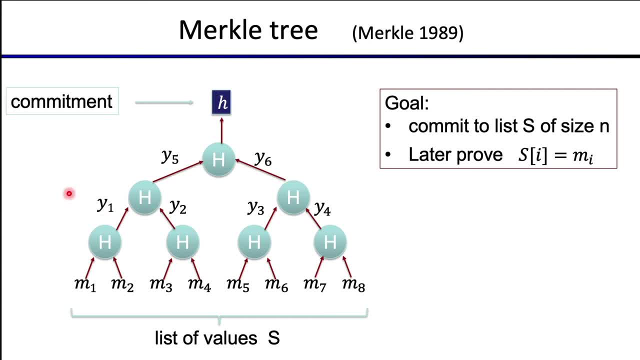 we'll call them y1,, y2, up to y6.. These are the internal hash values in the Merkle tree. And now let's suppose that we want to prove that S4 is equal to M4.. Okay, so we want to open up the fourth element in our list. 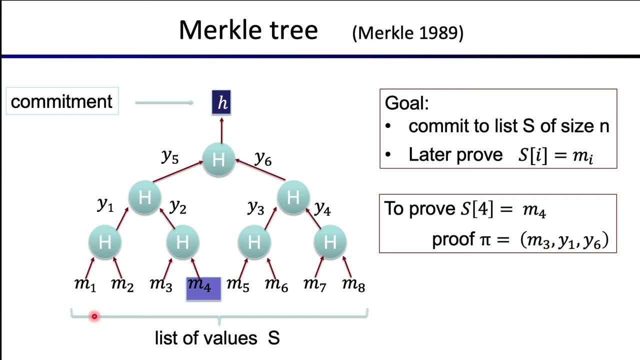 and then provide a proof that, in fact, M4 really is the thing that we committed to at position 4.. Well, the way we're going to do that is using the following proof. The proof is going to consist of the element M3, y1, and y6.. 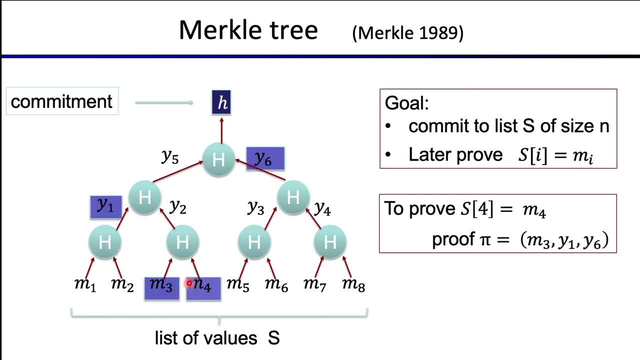 So let me show you what they are. So here are the elements, And what they are is really. you look at the path from M4 all the way to the root, And for each element along this path, you provide the sibling of that element. 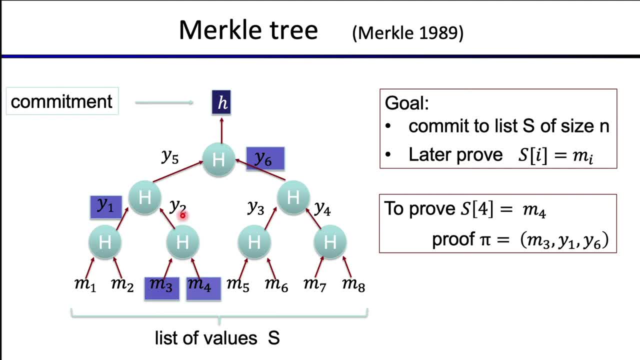 So for M4, we provide a sibling, namely M3.. For y2, we provide a sibling, namely M1.. And for y5, we provide a sibling, namely y6.. So the proof consists of these three elements. More generally, if we had a tree with N leaves, 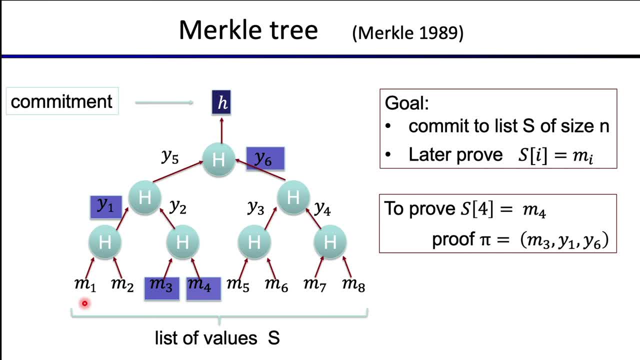 the depth of the tree would be log base 2 of N, So the proof would consist of log base 2 of N hashes, Which is really quite remarkable, because that means it's a really short proof. Think about a tree that contains a million elements. 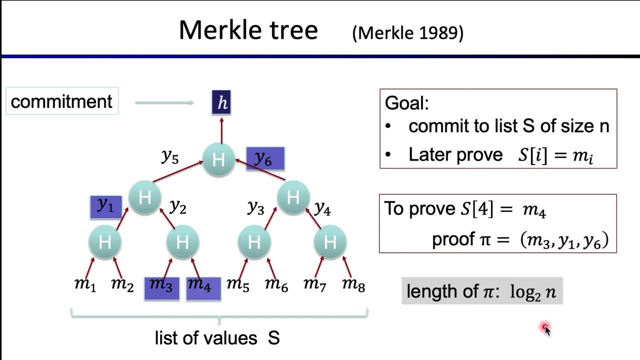 So imagine we're committing to a million elements. Well, log base 2 of a million is around 20.. So that means that the proof for proving that M4 is really what it's claimed to be, the proof, would only contain 20 hashes. 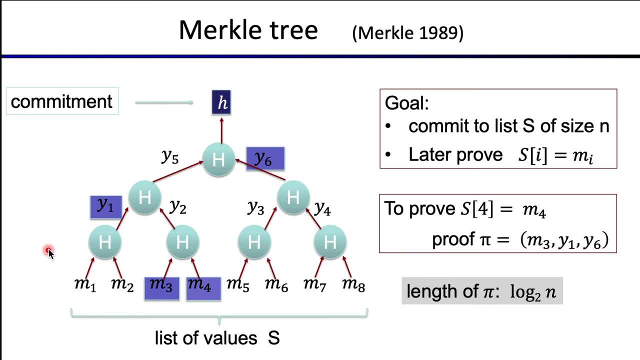 because log of a million is around 20.. Okay so, using a very short proof, we can prove that M4 is the value that's claimed. And now, how does Bob actually verify the proof? Okay, so, again, we want to prove that S4 is equal to M4.. 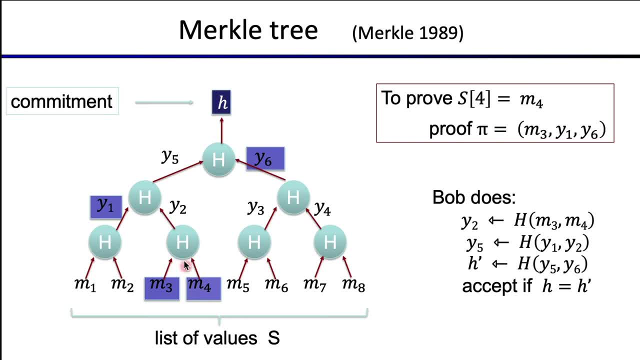 Well, what Bob would do is the following. It's kind of basically following up the path. So he would take the claimed M4 along with the element M3 from the proof and hash those together. That would give it a candidate for y2.. 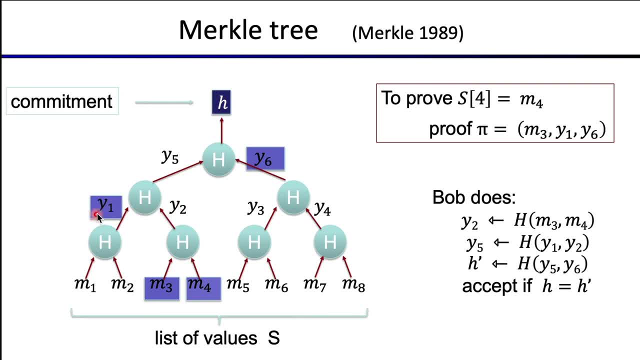 Then it would take y2 and hash it along with the element y1 from the proof. That would give it a candidate for y5.. It would take y5 and hash it along with y6 from the proof, And then y5 and y6 together. 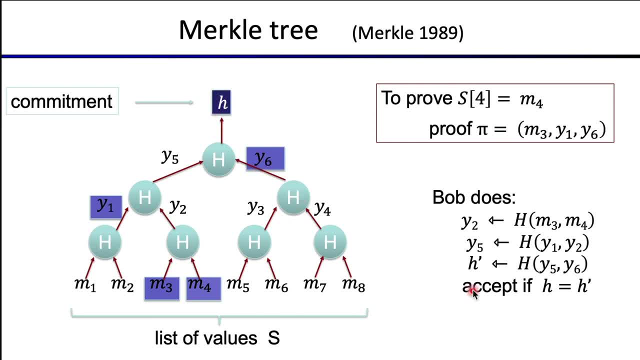 will give it a candidate h' for the Merkle output And then it will check. if h is equal to h' it will accept, otherwise it will reject. Okay, so not only is the proof contains only log n hash values, the verifier Bob can verify that the proof is correct. 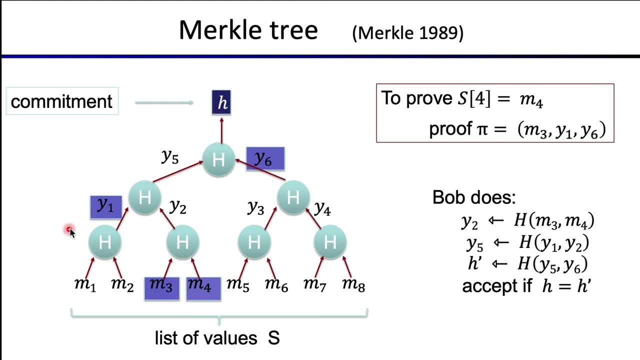 by literally computing only log n hashes. So very, very fast, Very fast verification of these Merkle proofs. Okay, so again very easy way to prove that a particular element in the committed set is what we claim it to be. So, in this case, M4 is the M4 that we claim it to be. 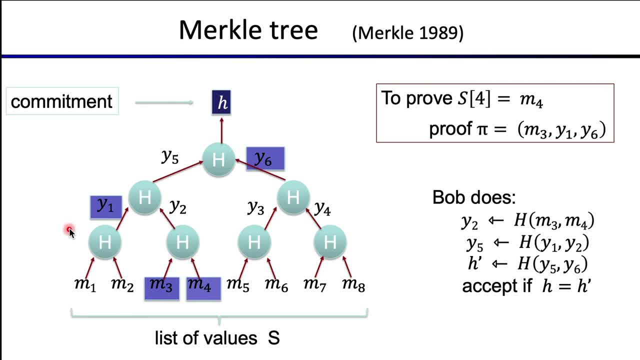 The proof contains only log n elements and it also only takes log n hash operations to verify this proof. Okay, so one last time. So Alice committed to a list of a million values. Well, in this case eight values, but in general. 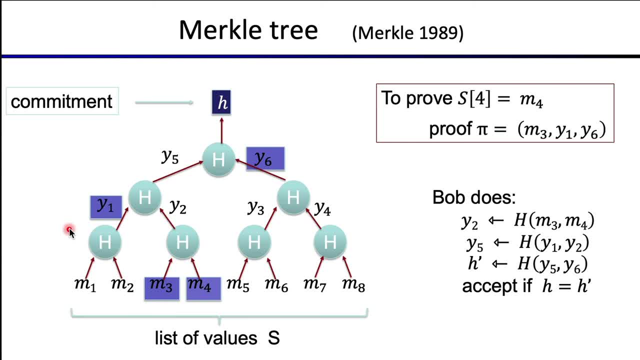 a very large list of values And then she can later open up any element in that list and prove that that element is consistent with the public commitment to the entire list. Yeah, again, in this case, h was the public commitment to the entire list. 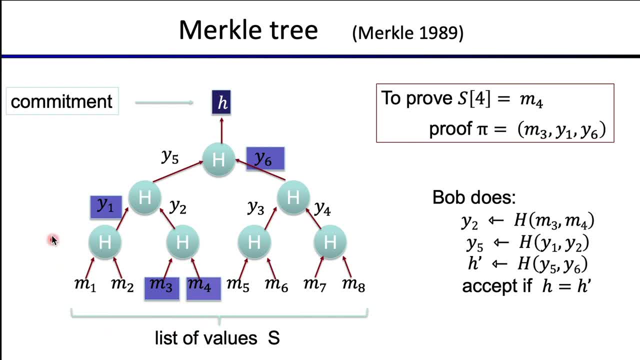 And Alice can prove that M4 is in fact the fourth element in the list that she committed to. And the proof is really short: It only contains three values and that's it. Okay, so you can prove a security, You can prove a security theorem that shows that this scheme. 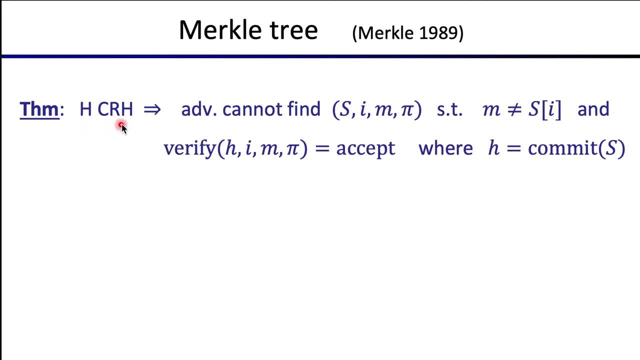 in fact is secure, In particular if h is a collision-resistant hash. it's fairly easy to prove that, in fact, the adversary cannot come up with a list S, an index i, a candidate M and a proof pi. 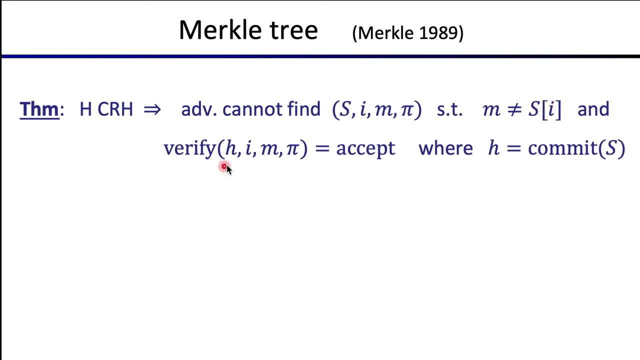 such that M is not the ith element in the list, And yet this verification procedure will accept M as if it were the ith element. This is actually a good exercise to try and prove yourself. If you want to prove this, try to prove the contrapositive. 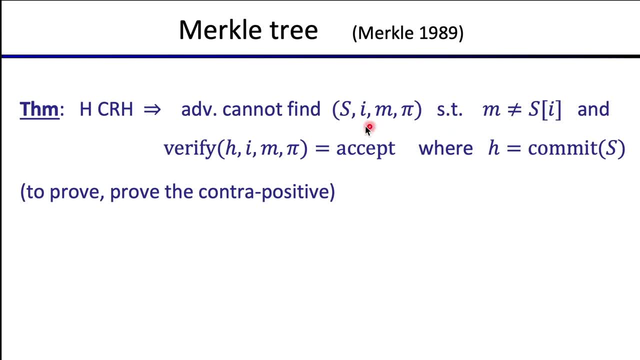 Namely, if Alice could come up with such a four-tuple, then she would be able to break collision-resistance of h. Yeah, it's a cute exercise to do, and I recommend that you try to prove this yourself. So what is this all useful for? 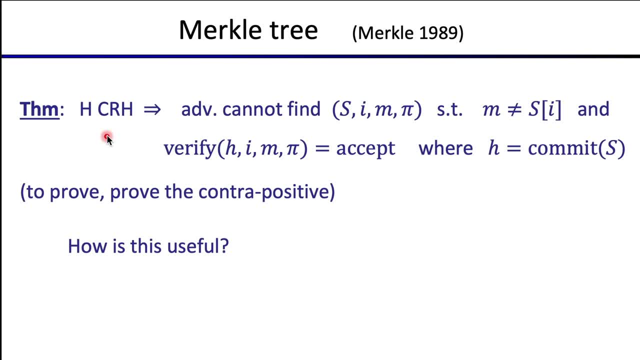 So we're able to commit to a large list of values and then later open a particular element in the list and prove that that element was opened correctly. Why is this useful? Well, it turns out it comes up all over the place, Yeah. 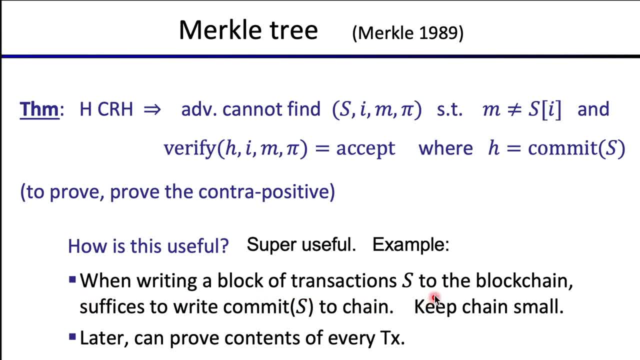 So, for example, when writing a block of code or a block of transactions, we're going to keep. the only thing we're going to write to the actual blockchain is going to be a commitment to the block of transactions. But later on, 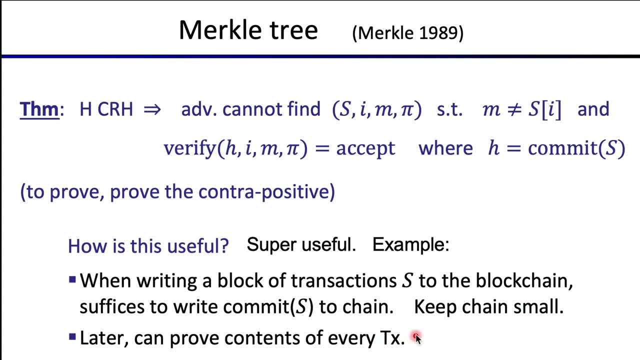 anyone can prove that any particular transaction is in the block by simply providing a Merkle proof that that transaction is included in that commitment. Okay, So it's an easy way to commit to a large list of transactions in a block using a very short commitment. 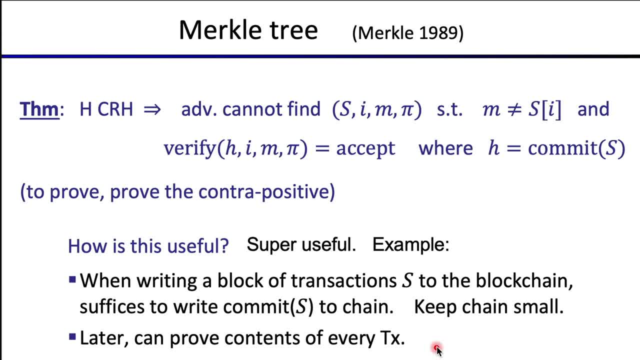 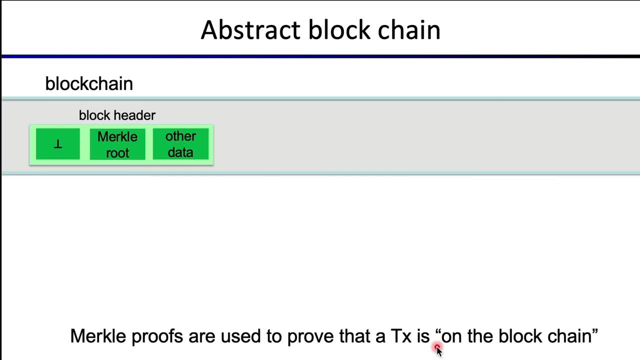 And if you're interested in a particular commitment in that block, you can actually prove that that commitment was included in that block. So really, when you think about what a blockchain is, it really is just a bunch of Merkle root commitments. Okay. 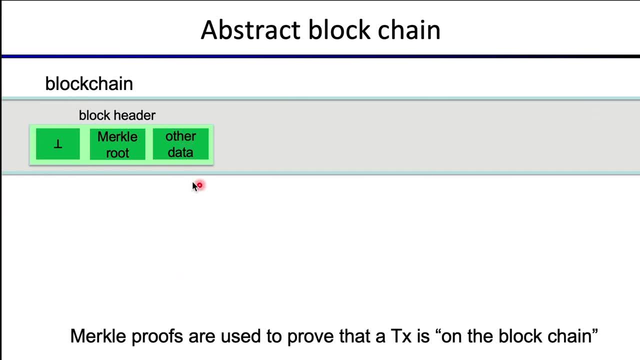 So really, a blockchain contains a bunch of block headers. So here you can see that there's a Merkle root commitment to a tree of transactions that are committed to in this block. Okay, but the block header really just includes the Merkle root. 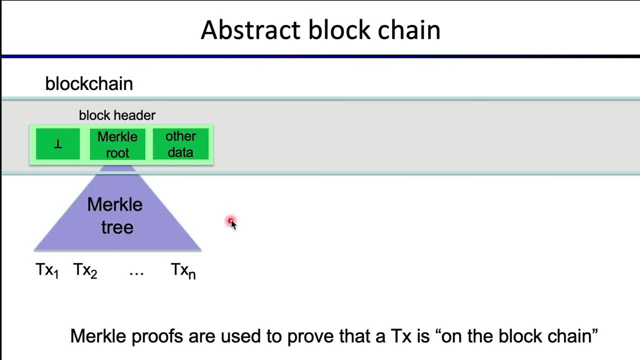 There's some other data which we won't get into, but that's not important. The main important thing here is that the block header contains a Merkle commitment to a list of transactions. The next block basically contains a hash of the previous block header.